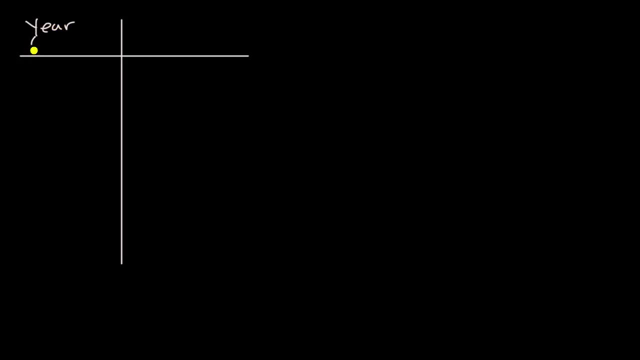 So let's say this is the year and we're gonna think about how much we have at the beginning of the year, and then this is the dollars in our account, And let's say that the bank is always willing to give us 5% per year, which is pretty good. 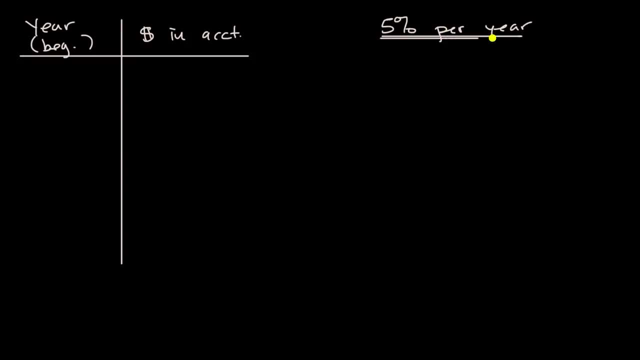 It's very hard to find a bank account that will actually give you 5% growth per year. So that means if you put $100 in at the end of a year or exactly a year later, it'd be $105.. If you put $1,000 in a year later, it'd be 1,050. 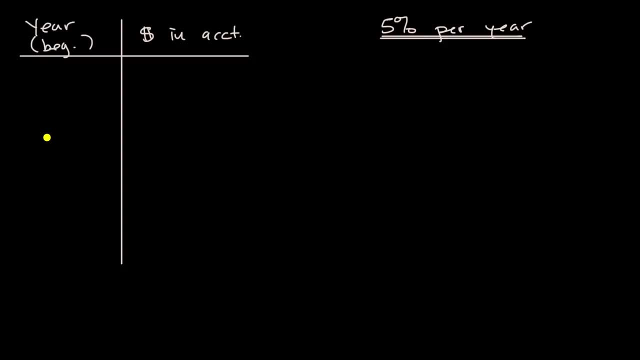 It'd be 5% larger. And so let's say that we wanna put $1,000 in per year and I wanna think about: well, what is going to be my balance at the beginning of year one, at the beginning of year two? 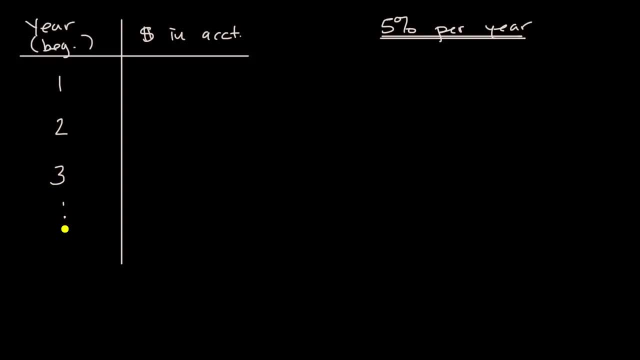 at the beginning of year three and then see if we can come up with a general expression for the beginning of year N. So year one, right at the beginning of the year, I put in $1,000 in the account. That's pretty straightforward. 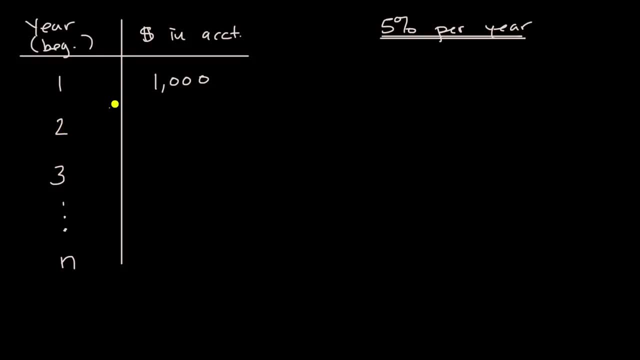 But then what happens in year two? I'm going to deposit $1,000, but then that original $1,000 that I have would have grown. So I'm going to deposit $1,000, and then the original $1,000,. 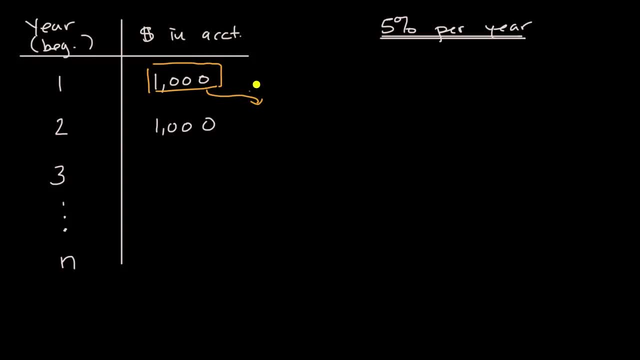 that I put at the beginning of year one that is now grown by 5%. Growing by 5% is the same thing as multiplying by 1.05.. So this is now going to be plus $1,000 times 1.05.. 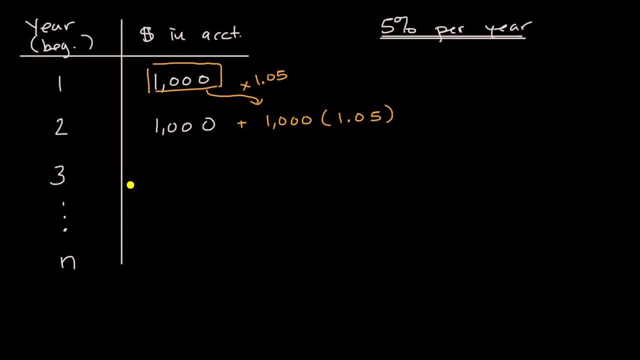 Fairly straightforward. Now, what about the beginning of year three? How much would I have in the bank account right when I've made that first, that year three deposit? Pause this video, see if you can figure that out. Well, just like at the beginning of year two. 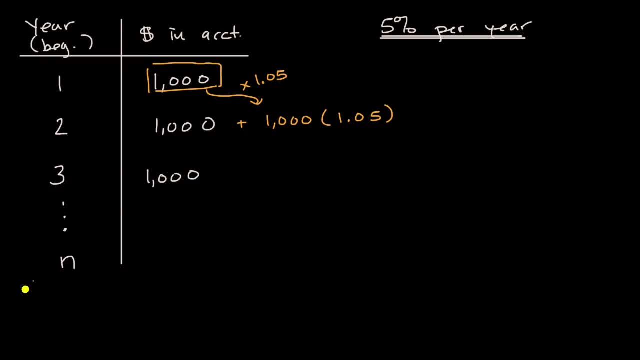 and the beginning of year one, we're going to make a $1,000 deposit, But now the money from year two has grown by 5%, So this is now going to be $1,000 times 1.05.. And then that money that we originally deposited. 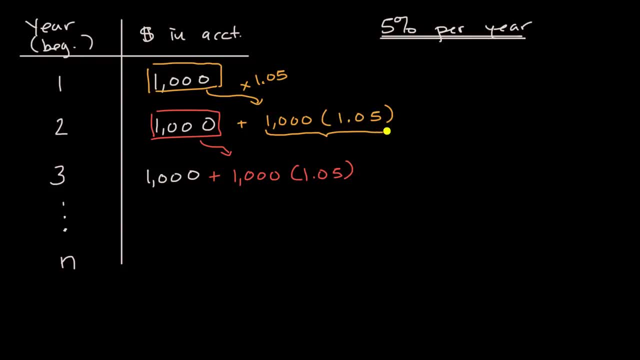 from year one that was 1,000 times 1.05. in year two that's going to grow by another 5% And so this is going to be 1.05.. So this is going to be plus 1,000 times 1.05 times 1.05.. 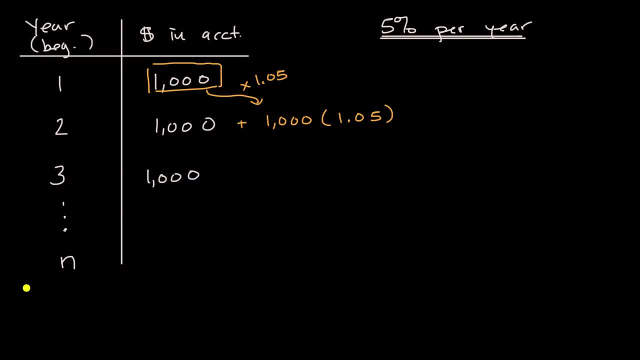 and at the beginning of year one we're gonna make $1,000 deposit, But now the money from year two has grown by 5%, So this is now going to be $1,000 times 1.05.. And then that money that we originally deposited. 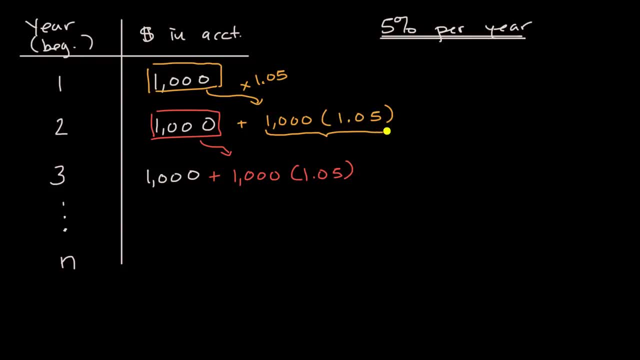 from year one that was $1,000 times 1.05. in year two That's going to grow by another 5%. So this is going to be plus 1,000 times 1.05, times 1.05.. 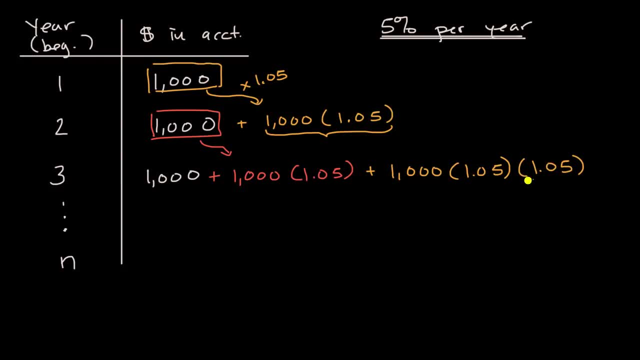 We're going by another 5%. Well, we could just rewrite this part right over here as 1.05 squared. So do you see a general pattern that's going to happen here? Well, as you go to year n, in fact, pause the video again. 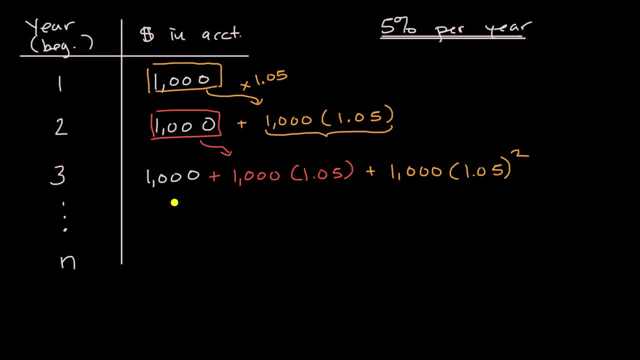 and see if you could write a general expression. You're going to have to do a little bit of this dot dot dot action in order to do it, but see if you could write a general expression for year n. Well, for year n you're going to make. 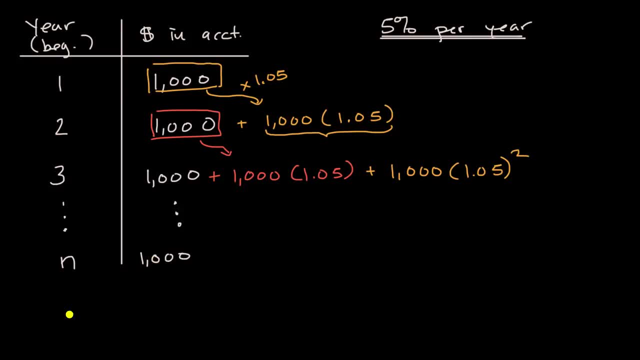 that original $1,000 at the beginning of year n, and then you're going to have 1,000 times 1.05 for that $1,000 that you deposited at the beginning of year n, minus one, and then this is just going to keep going. 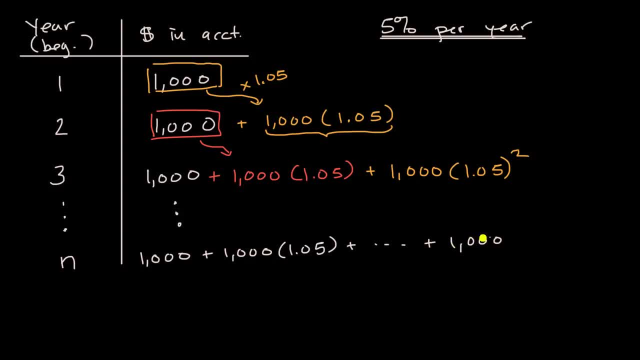 and it's going to go all the way to plus $1,000 to times 1.05 to the power of the number of years you've been compounding. So you could view this $1,000 as the one that you put in year one. 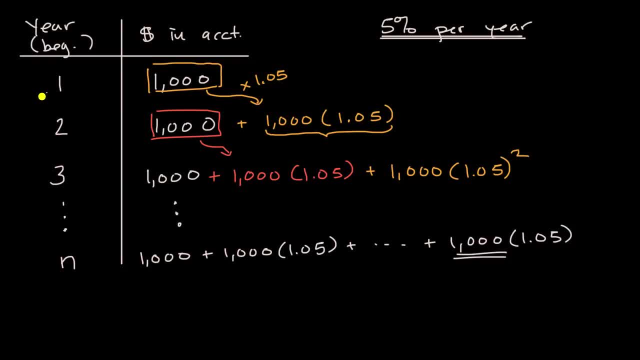 and then, how many years has it compounded? Well, when you go from one to two, you've compounded one year. When you go from one to three, you've compounded two years. So, when we're talking about the beginning of year n, 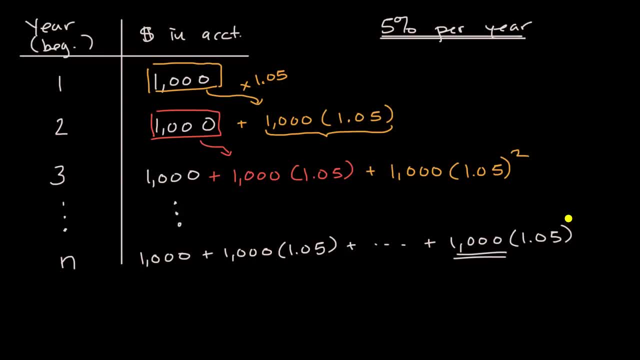 you go up to the exponent that is one less than that, and so this is going to be to the n minus one power. So what we just did here is we've just constructed each one of these When we're saying: okay, how much money do we have? 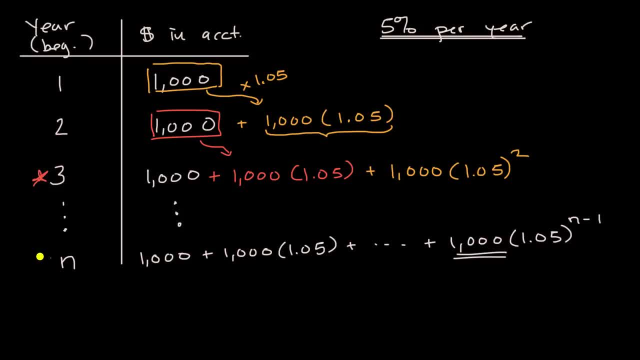 in our bank account at the beginning of year three, or how much do we have in our bank account at the beginning of year n? these are geometric series, and now I'll write that word down: Geo geometric series. Now, just as a little bit of a review. 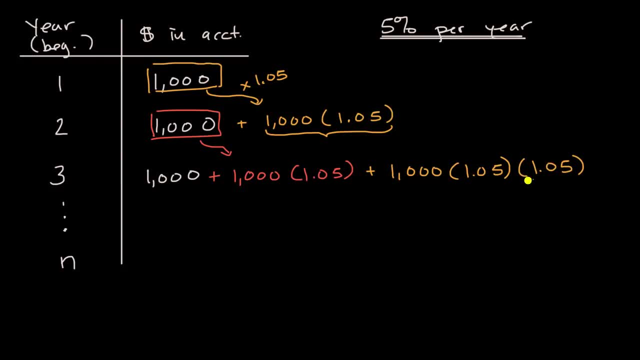 We're going by another 5%. Well, we could just rewrite this part right over here as 1.05 squared. So do you see a general pattern that's going to happen here? Well, as you go to year n, in fact, pause the video again. 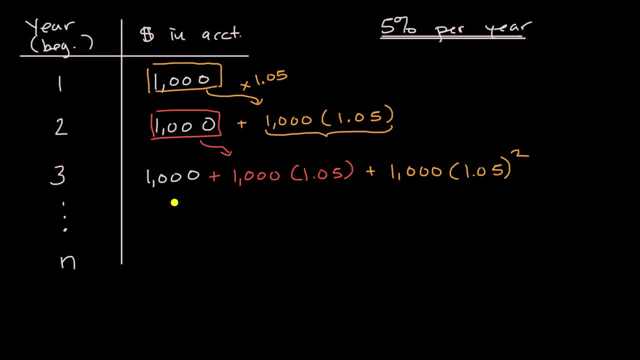 and see if you could write a general expression. You're going to have to do a little bit of this dot dot dot action in order to do it, but see if you could write a general expression for year n. Well, for year n you're going to make. 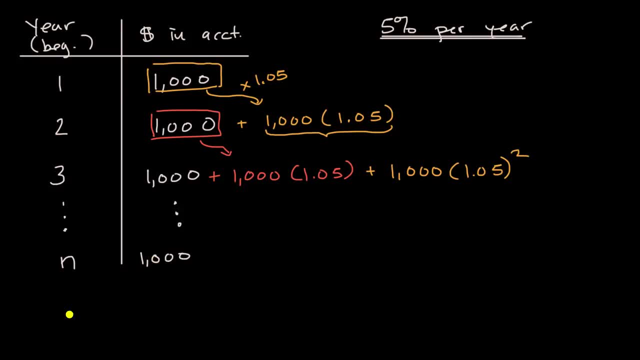 that original $1,000 at the beginning of year n, and then you're going to have 1,000 times 1.05 for that $1,000 that you deposited at the beginning of year n, minus one, and then this is just going to keep going. 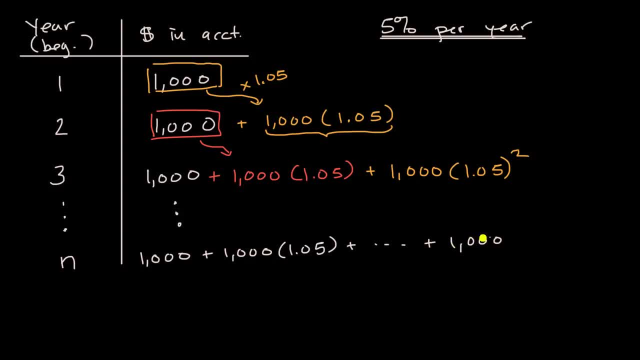 and it's going to go all the way to plus $1,000 to times 1.05 to the power of the number of years you've been compounding. So you could view this $1,000 as the one that you put in year one. 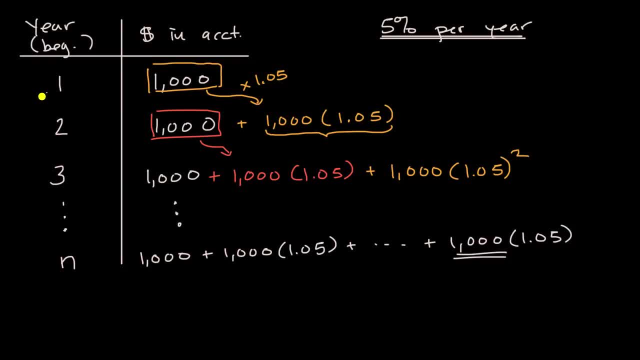 and then, how many years has it compounded? Well, when you go from one to two, you've compounded one year. When you go from one to three, you've compounded two years. So, when we're talking about the beginning of year n, 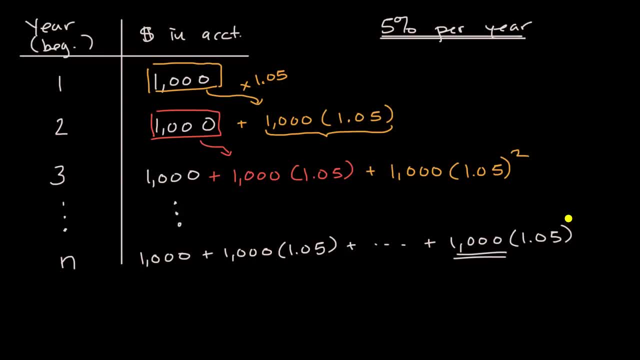 you go up to the exponent that is one less than that, and so this is going to be to the n minus one power. So what we just did here is we've just constructed each one of these When we're saying: okay, how much money do we have? 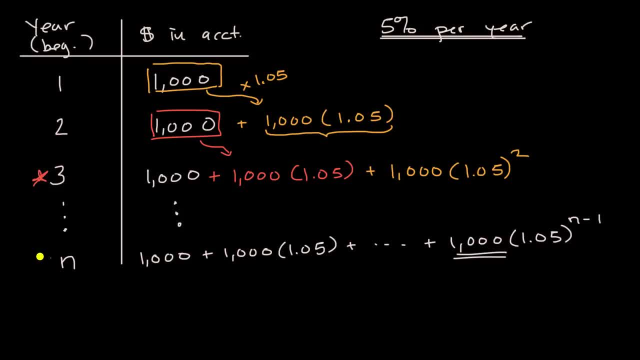 in our bank account at the beginning of year three, or how much do we have in our bank account at the beginning of year n? these are geometric series, and now I'll write that word down: Geo geometric series. Now, just as a little bit of a review. 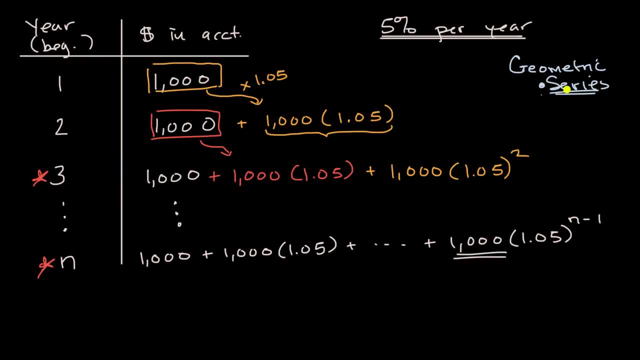 or it might not be a review, it might be a primer. series are related to sequences and you can really view series as sums of sequences. So a sequence is- and let me go down a little bit so that you can. so we have a little bit more space. 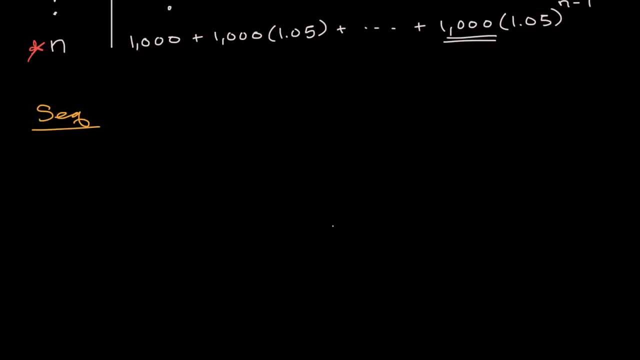 A sequence is an ordered list of numbers. A sequence might be something like: well, let's say we have a geometric sequence. In a geometric sequence, each successive term is the previous term times a fixed number. So let's say we start at two. 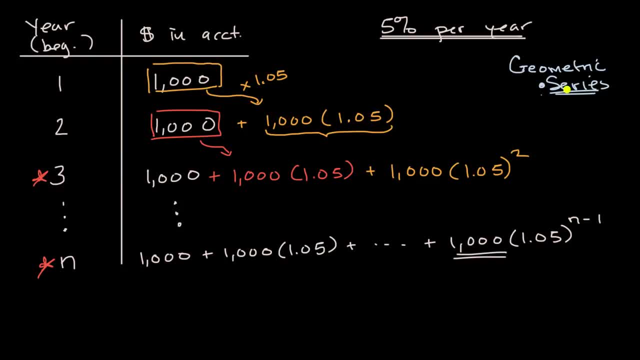 or it might not be a review, it might be a primer. series are related to sequences and you can really view series as sums of sequences. So a sequence is- and let me go down a little bit so that you can. so we have a little bit more space. 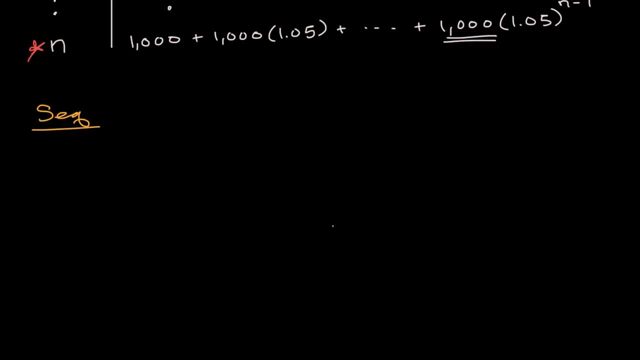 A sequence is an ordered list of numbers. A sequence might be something like: well, let's say we have a geometric sequence. In a geometric sequence, each successive term is the previous term times a fixed number. So let's say we start at two and every time. 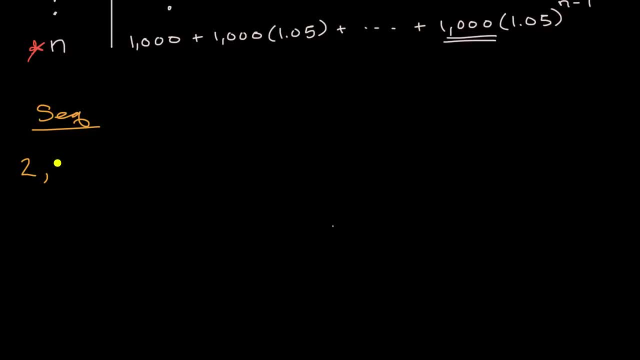 we multiply by three. So we'll go from two. two times three is six. six times three is 18.. 18 times three is 15.. 18 times three is 15.. 18 times three is 54.. This is a geometric sequence. ordered list of numbers. 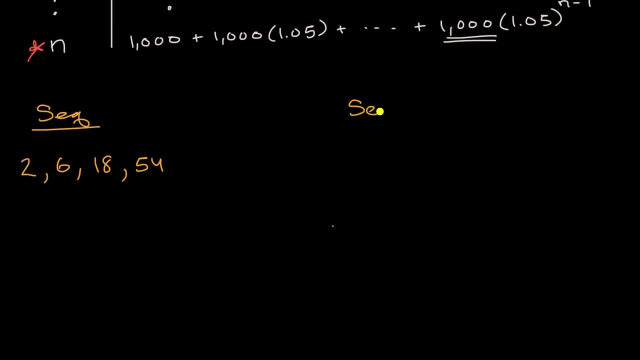 Now, if we want to think about the geometric series or the one that's analogous to this, is that we would sum the terms here, So this would be two plus six, plus 18 plus 54. Or we could even write it and this will look similar. 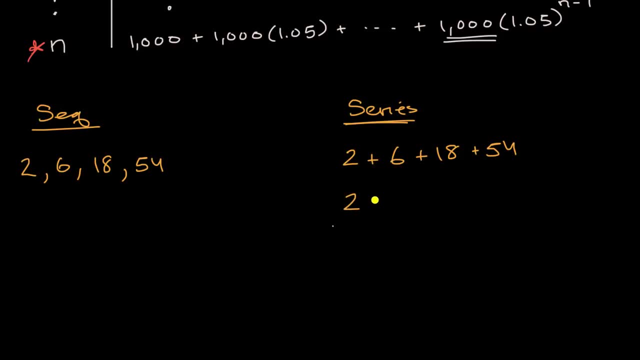 to what we had just done with our little savings. example is: this is two plus two times three plus two times three squared, plus two times three to the third power, And so, with a geometric series, you're going to have a sum where each successive term 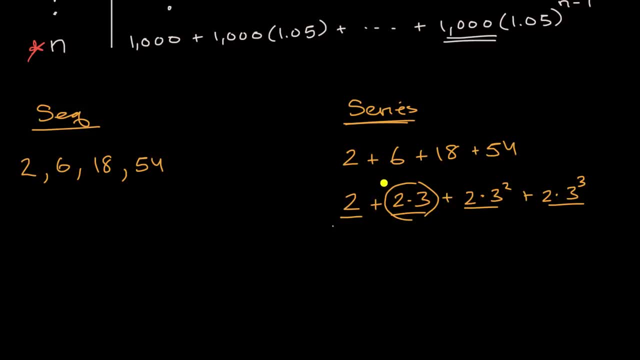 in the expression is equal to. if you put them all in order, is going to be equal to the term before it times a fixed amount. So the second term is equal to the first term times three and we're summing them In a sequence. you're just looking at it. 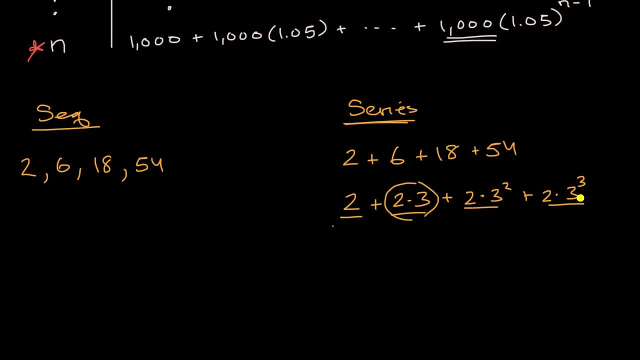 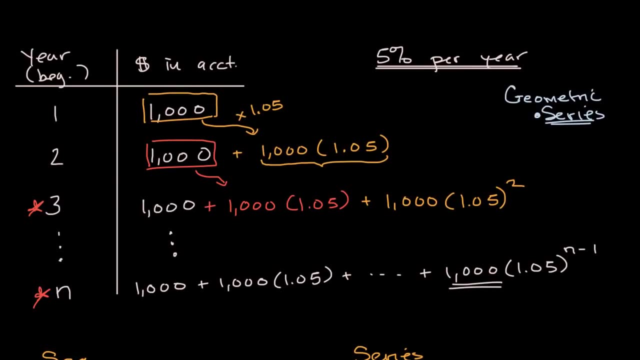 It's an ordered list, so to speak, but here you are actually adding up the order. It's an ordered list. So what we just saw in this example is why a one what a geometric series is, but also a famous example of how it's useful. 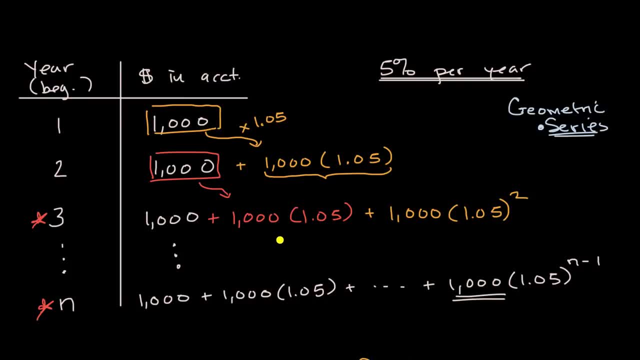 and this is just scratching the surface. If you were to go further in finance or in business, you'll actually see geometric series popping up all over the place.